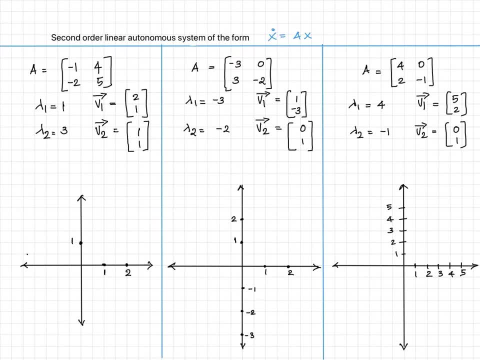 We consider three different cases of real eigenvalues. Let us start with both positive eigenvalues For which capital A is selected as minus 1, 4, minus 2, 5. We can see that the eigenvalues of the system are lambda 1 equal to 1 and lambda 2 equal to 1.. 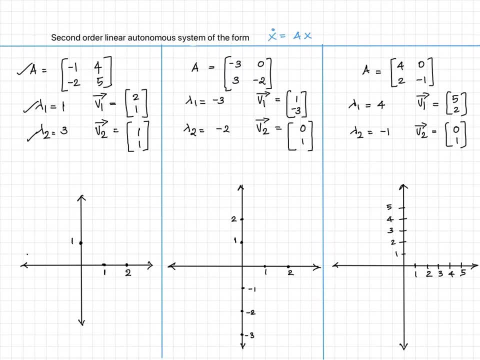 For which the eigenvectors are respectively 2, 1 and 1: 1.. As far as second order linear systems are concerned, the singular point is x1 equal to 0 and x2 equal to 0. It is a unique singular point. 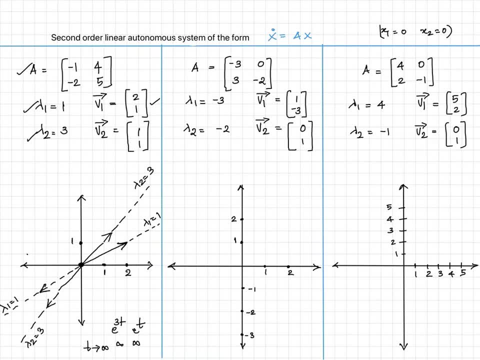 If you look at the eigenvectors, we can see that the eigenvector corresponding to lambda 1 equal to 1 would be like this, And the eigenvector corresponding to lambda 2 equal to 3 would be like this, Since the modes of operation corresponding to the eigenvalues are e raised to 3t and e raised to t. 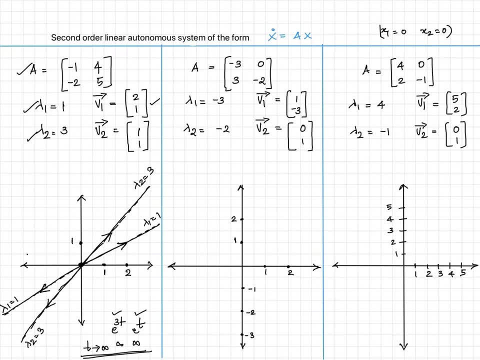 And as t tends to infinity, these values tend to infinity, We can say that the solutions will move away from the equilibrium point. So In this case, if you consider a phase trajectory, we can see that the component of e raised to 3t would be larger than e raised to t. 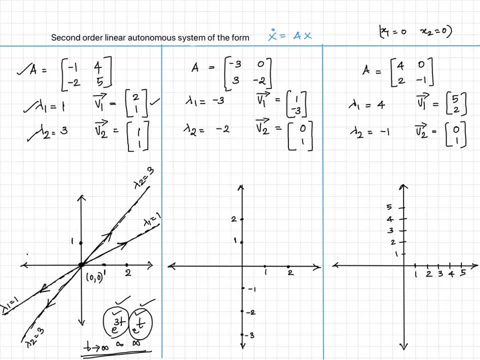 The trajectories will start along lambda 1, equal to 1 line, and then move towards lambda 2, equal to 3 lines, In both the sections. With other initial conditions it would be like this, That is, it moves parallel towards lambda 2, equal to 3 line, as t tends to infinity. 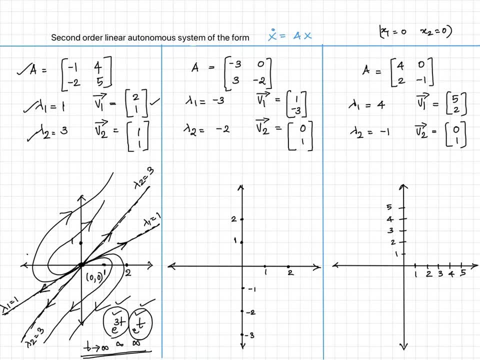 If you consider the region between the eigenvalues, it would be like the phase trajectories would start with lambda 1, equal to 1 line, and then move towards lambda 2, equal to 3 line. Such a phase trajectory makes no sense, So we don't consider the phase trajectories in between these two sections. 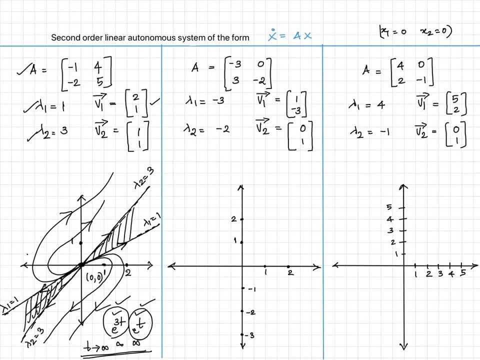 That is here and here. If you consider any other phase trajectory, it would be something like this: Since the phase trajectories move away from the equilibrium point, we stay the equilibrium point or singular point, as an unstable node. Now we consider the case when the eigenvalues are negative. 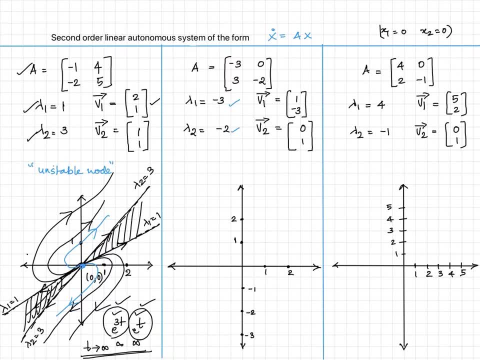 Here the first eigenvector is 1 minus 3.. And the second eigenvector is 3.. So this corresponds to lambda 1 equal to minus 3, and this corresponds to lambda 2 equal to minus 2.. Since both the eigenvalues are negative, the solutions will have e raised to minus 3t and e raised to minus 2t. 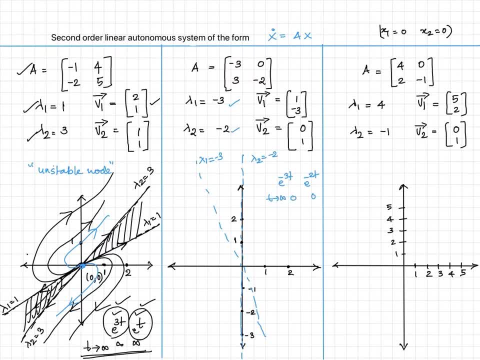 Which tend to 0, as t tends to infinity. Hence we can say that the solutions move towards the origin along this line. So, with different initial conditions, The phase trajectories would move parallel to these lines. So we shall consider a phase trajectory, initially starting parallel to e raised to minus 3t line and then tending towards the origin parallel to e raised to minus 2t line. 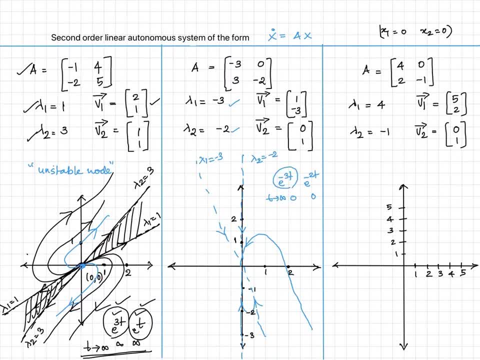 This is because e raised to minus 3t decays faster than e raised to minus 2t. So by the time t tends to infinity, e raised to minus 2t term will be present. And if you consider the other case, we can see. it is something like this: 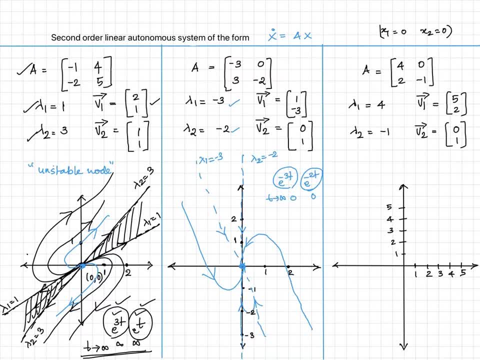 So, since the phase trajectories move towards the singular point, we call this as a stable node. So the phase trajectories would be like this: If you consider the region in between, the phase trajectories would make no sense. It would be something like this: 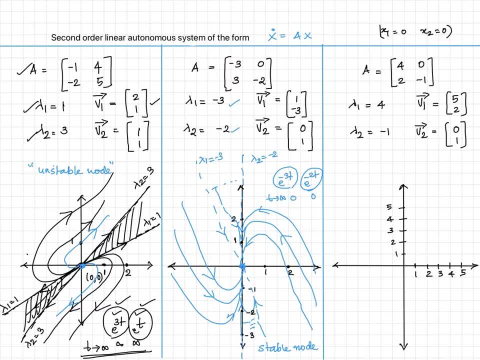 Now we consider the case when the eigenvalues are different, That is, one positive and one negative. In this case, the eigenvector would be 5, 2. And 0, 1.. So this corresponds to lambda equal to 4 and this corresponds to lambda equal to minus 1.. 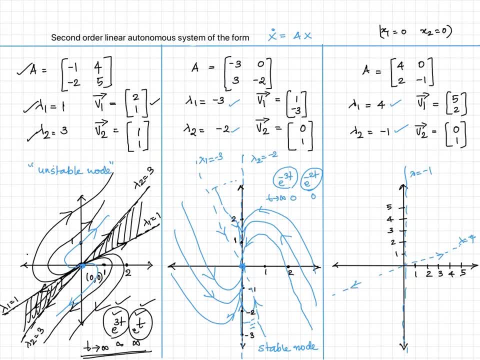 Since this is a positive eigenvalue, the eigenvectors would be moving away and the solution would be moving away, Whereas here, the solutions will be moving towards the equilibrium point And the modes of cooperation would be e raised to 4t and e raised to minus t. 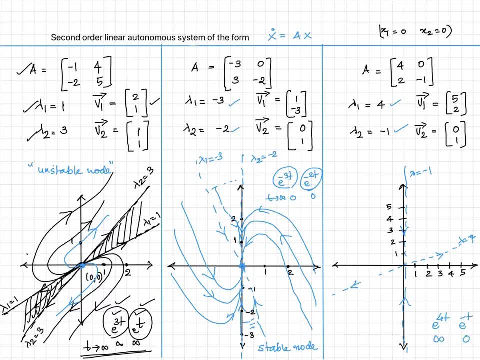 As t tends to infinity, this term tends to infinity and this term tends to serve. So the phase trajectories would start with e raised to minus t term and ends with e raised to 4t term. So all phase trajectories would start parallel to e raised to minus t and move parallel to e raised to plus 4t. 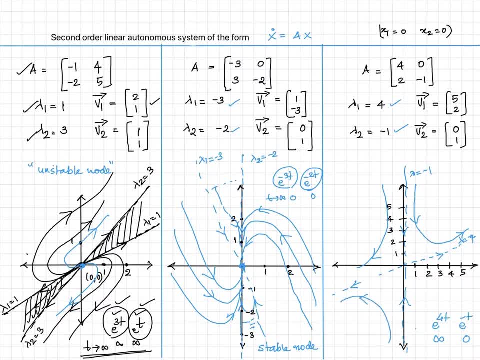 So in the various regions, the phase trajectories could be marked like this: Since this takes the shape of a saddle, the equilibrium point is said to be a saddle. We can see that initially it appears to be stable because it is moving towards the equilibrium point. 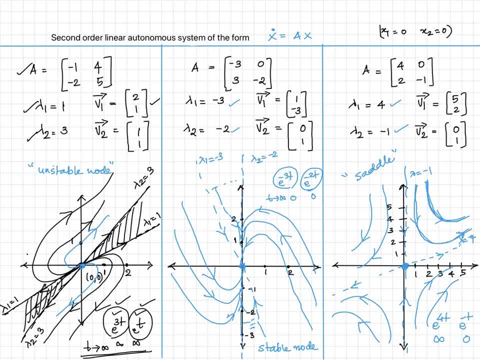 But later it tends to move away from the equilibrium point. So here I consider the case when the eigenvalues are different. So in the various regions the phase trajectories would start with e raised to minus t term and ends with e raised to minus t. 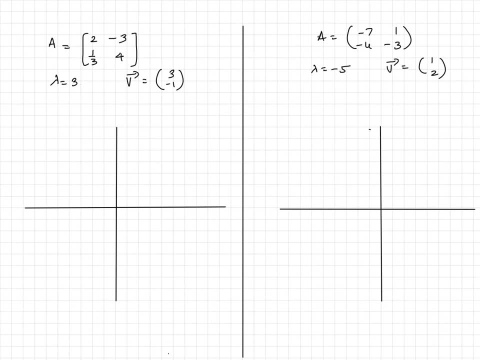 So in this case the eigenvalues are same, Either both positive or both negative. So in this case I take an example for a matrix like this: That is 2 minus 3, 1 by 3, 4.. 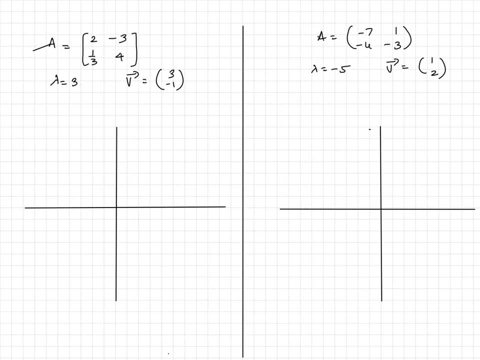 The eigenvalues are 3, 3.. I find the eigenvector corresponding to one of the eigenvalues. It appears to be 3 minus 1.. So this will be the eigenvector line. Since the eigenvalue is positive, we can see that the solutions will be moving away from the equilibrium point. 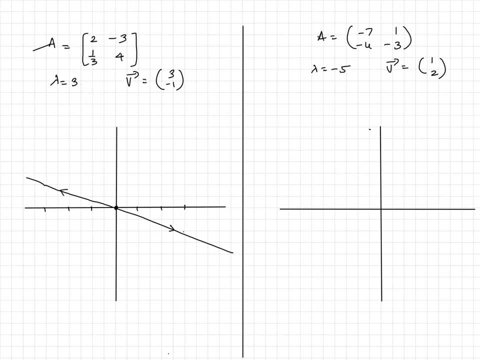 from the singular point. Now, in order to draw the phase trajectory, we should identify the direction. Here we have only one set of eigenvectors, So a simple trick is you just find some vector and see whether the resultant of this vector with the system matrix is moving. 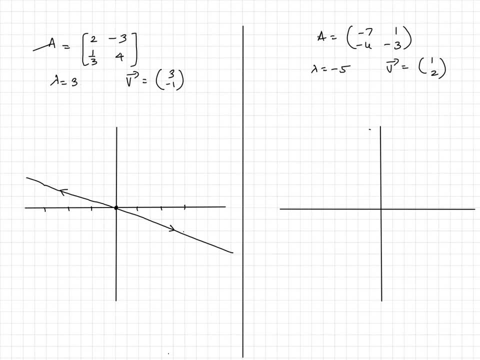 in the clockwise or counterclockwise direction. For example, I take a vector 0, 1.. I just multiply this by 2 minus 3,, 1 by 3, 4, and the resultant is minus 3, 4.. So it shows. 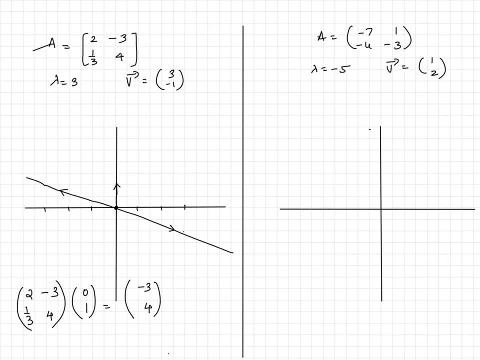 that any vector 0, 1 will be moving towards minus 3, 4 once multiplied by this A matrix, This shows that the vector movement is in the counterclockwise direction. This is the phase trajectory. This shows that all the phase trajectories starting along one of the 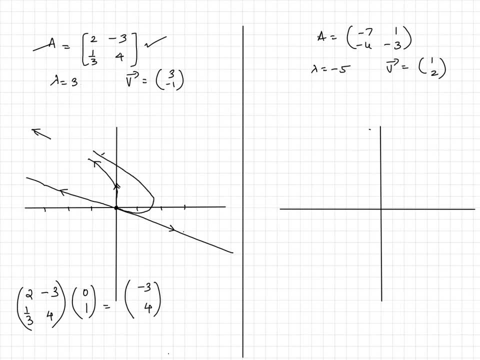 eigenvector line will be moving in the counterclockwise direction. So the phase trajectories will be moving in the counterclockwise direction And since the eigenvalue is positive, it moves away from the singular point. This is also a case of unstable node. Now consider a case. 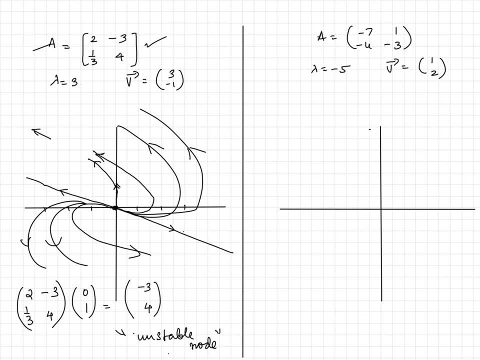 for a negative eigenvalue. So in this case the eigenvector is 1, 2.. So I can mark the eigenvector line as 1, 2.. And since the eigenvalue is negative, the solutions will be moving towards the singular. 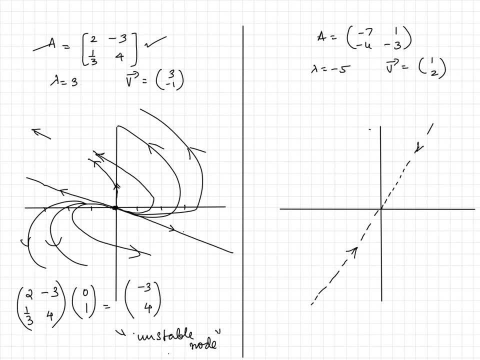 point. Now we need to find the direction of the phase portrait, for which I take an example: 1, 0, any vector multiplied by the system matrix, I get the result as minus 7, minus 4.. So 1, 0 is a vector like this, Minus 7, minus. 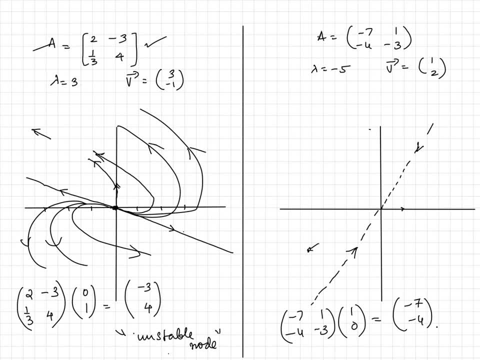 4 would be something here around this. So this shows that it is moving in this direction from 1, 0 to minus 7, minus 4, which means the phase trajectories are moving in the clockwise direction. So any phase trajectory running parallel to this part would tend towards the. 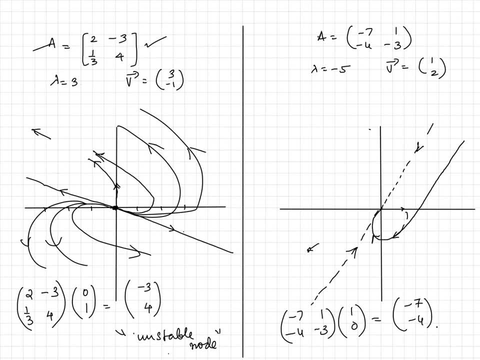 origin Parallel to the other part. So here also it would be something like this. So here we have phase trajectories moving towards the singular point. This is also an example of a stable node: singular point. Now we consider the cases for complex eigenvalues. 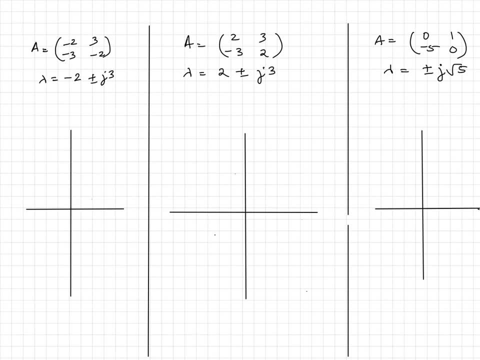 In the case of complex eigenvalues, we consider the real part and then identify whether these phase trajectories would be moving towards the equilibrium point or away from the equilibrium point. In the first case we have a negative real part. So in that case the phase trajectories 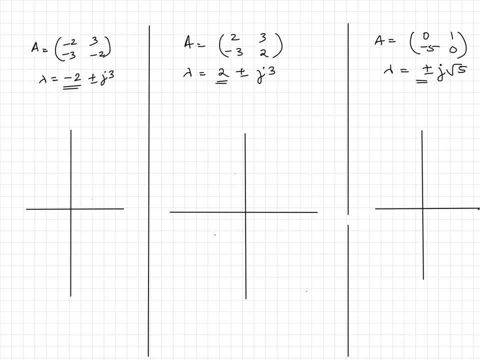 will be moving towards the equilibrium point. In order to find the direction of the phase trajectory, we just use the previous example. So in the first case we have a negative real part. Let us define this in the previous row, That is, we consider any vector multiplied. 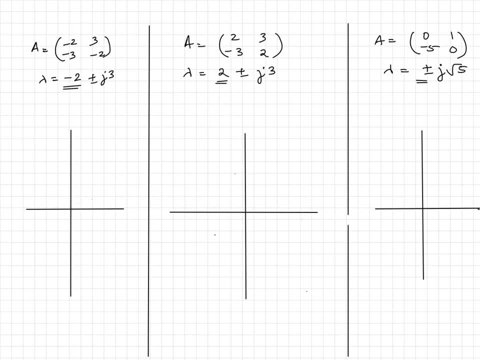 by capital A and see how the direction occurs. So we consider a vector 1, 0 multiplied by minus 2, 3 minus 3 minus 2.. That is a system matrix that results in minus2 minus3.. So 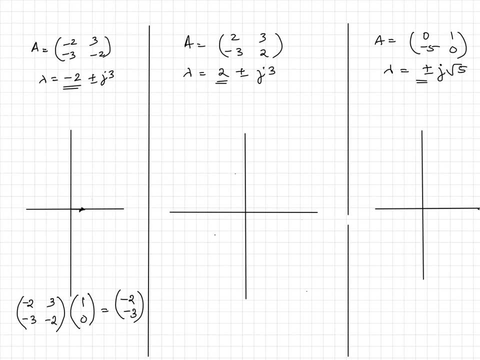 a vector 1,0 when multiplied by the system metrics will be given the teenagers for once –1.. So Agora, let us consider this in aты testimolar form. Once the behavior Anytime look at this system matrix results in minus 2, minus 3.. So it means that the vector should move in. 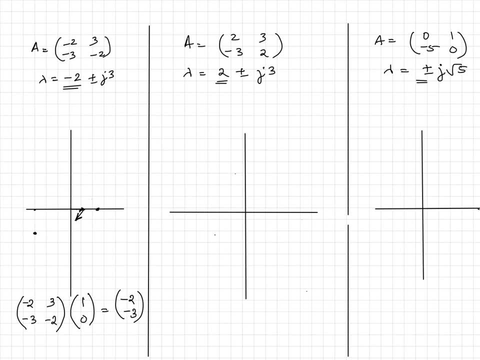 this direction. So if you have an initial point like this, then the phase trajectory would be tending towards the origin. in this way The singular point is called a stable focus. Next, we consider the case for a positive real part for the eigenvalue. Here again we 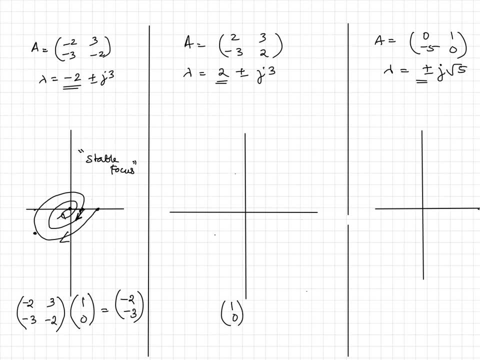 consider the same vector 1, 0 and see the direction of the phase trajectory. with the help of this vector, We multiply the system matrix and get a result as 2 minus 3.. So if you consider a vector 1, 0, the resultant